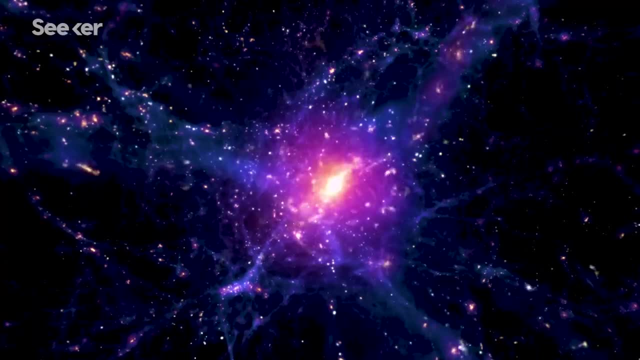 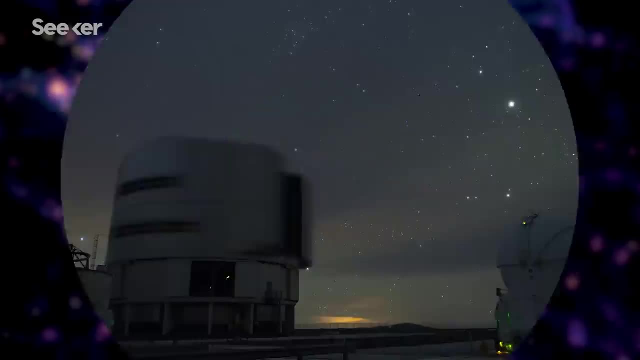 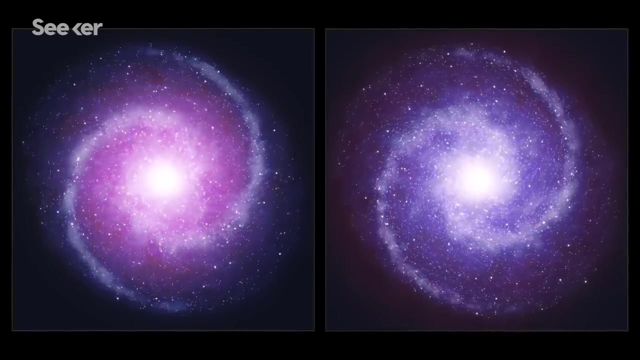 This is like setting a musical scale. You're listening for what would sound kind of like a tone amidst a sea of white noise. There's numerous astrophysical measurements that look at things in the universe. There are things out there that are interacting gravitationally. 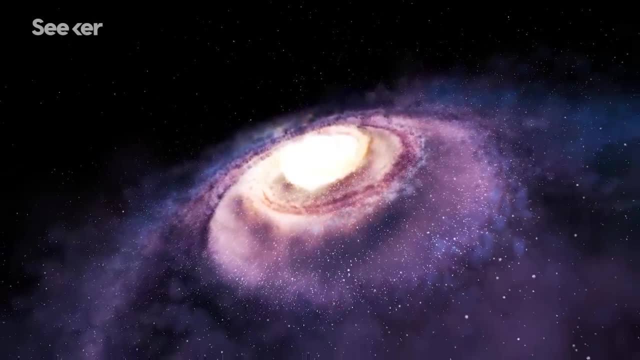 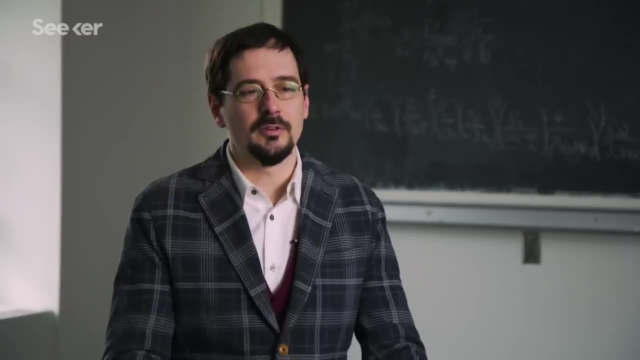 That aren't stars, They don't seem to be dust, They're not planets, as far as we can tell. You find that this extra stuff out there isn't even made of atoms. This is very peculiar, because you're made of atoms, I'm made of atoms. 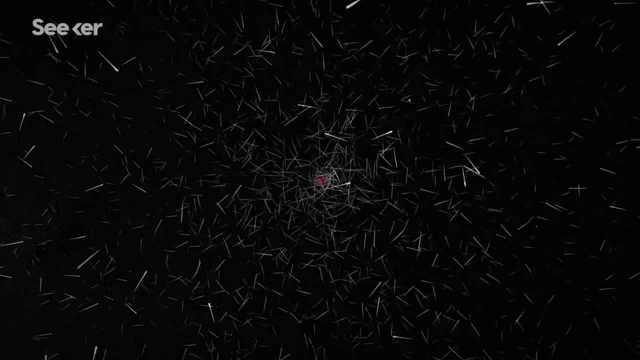 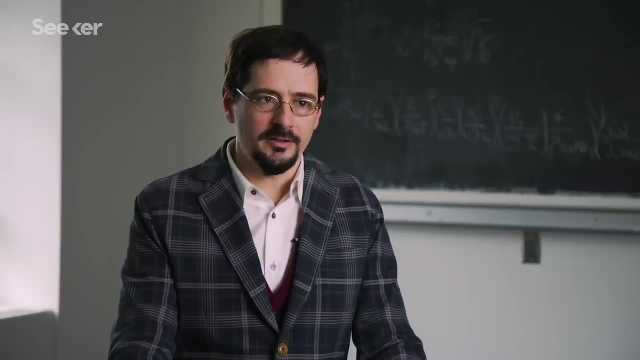 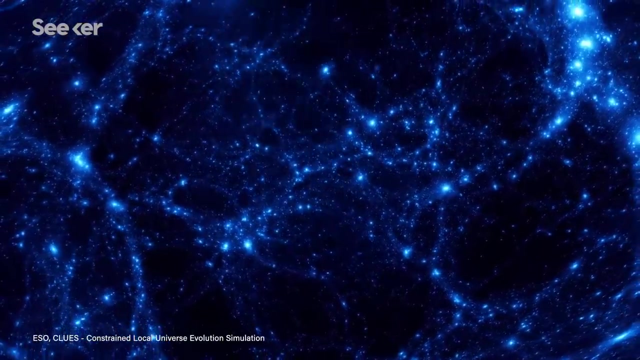 Almost everything we can study is made out of atoms, and so this means there's something new and different out there, some new, different particle, and we call it dark matter. So the theorist sees these astrophysical observations and says, aha, there's something new out there and they've got a set of things that could. 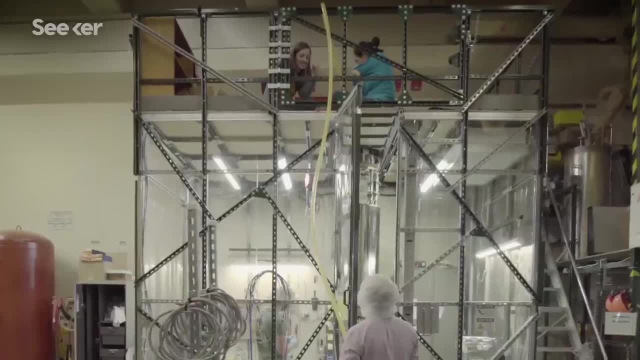 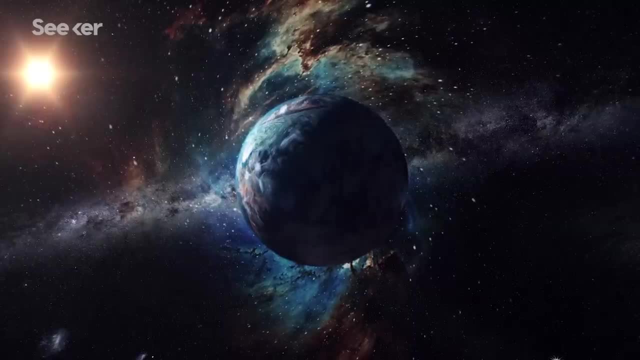 could exist but don't necessarily do exist, And the experimentalist's job is basically to go through these one at a time. On the list are some dark matter particles with names as weird and curious as the physics behind them. People have heard of WIMPs. 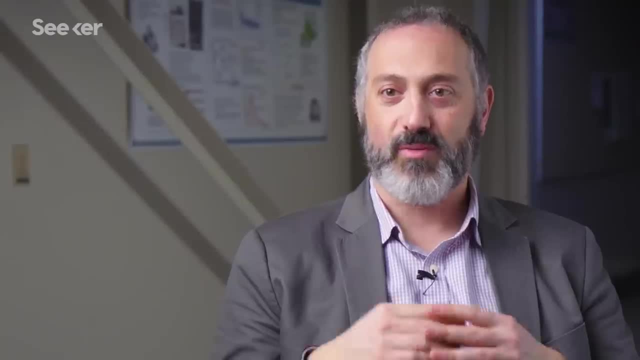 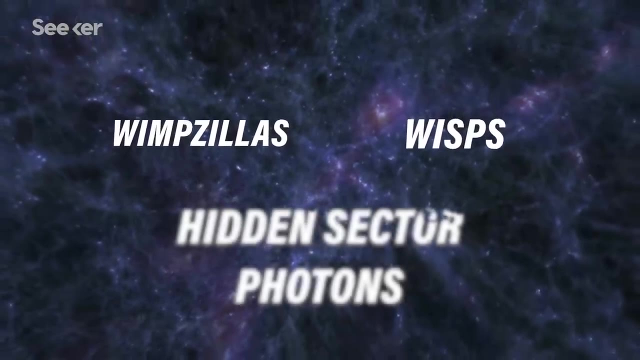 There's also MACHOs, which is kind of the exact opposite of a WIMP. Those are massive astronomical compact halo objects, Think black holes. There's WIMPzellas, WISPs, hidden sector photons. There's stealth dark matter. And the star of this episode that's going to be the star of this episode is going to be the star of this episode, And the star of this episode that's going to be the star of this episode is going to be the star of this episode. 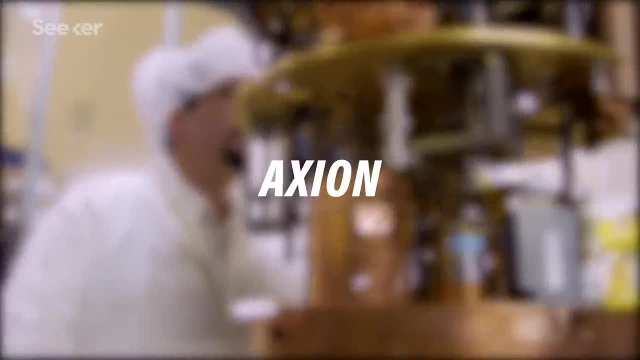 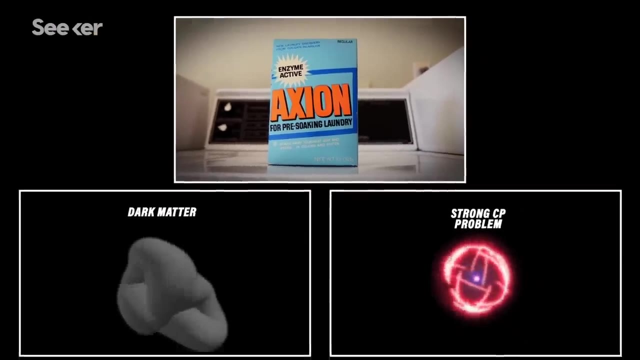 And the star of this episode that's going to be the star of this episode is going to be the star of this episode. This big experimental push is called the axion. This theoretical particle was named after laundry detergent in the 1970s because it could clean up two big problems in physics. 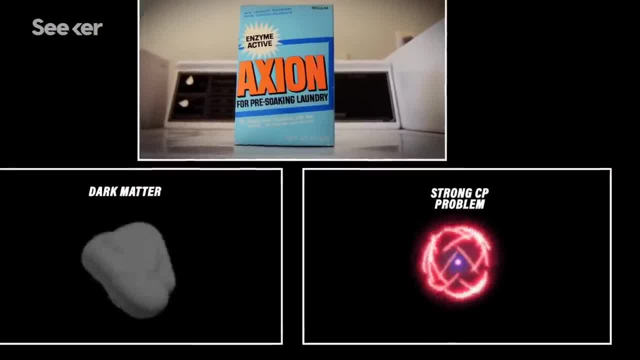 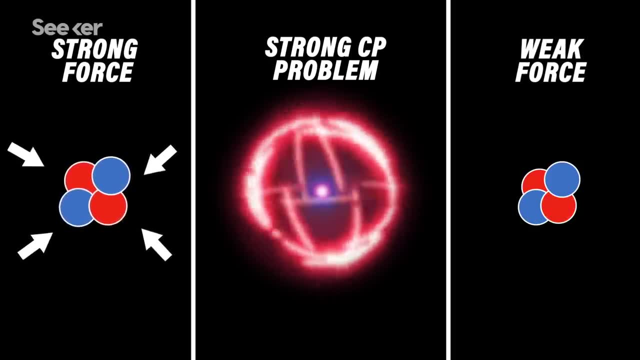 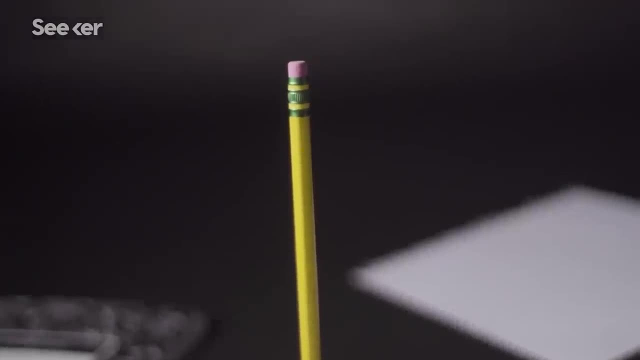 dark matter and the strong CP problem. This is another perplexing mystery that involves a surprising balance between two of the fundamental forces of nature: the strong force and the weak force. One way to think about it simply is: If you see a pencil that's kind of just sitting there on its head. 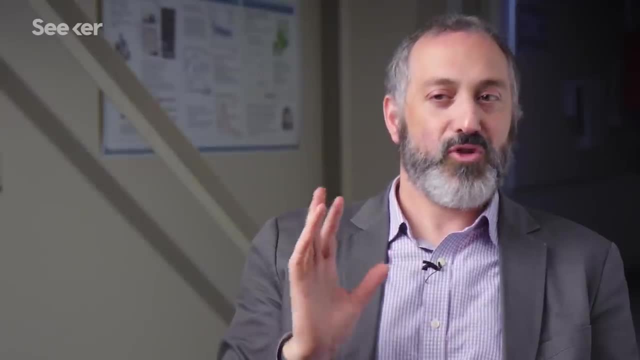 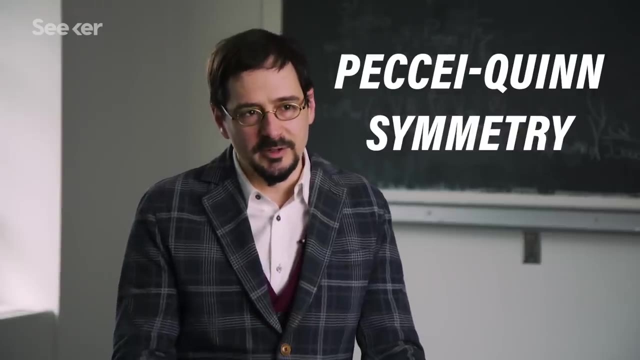 and not falling over. that's strange. It should fall over unless something else is holding there. The best idea for that is something called Pecet-Quinn symmetry, which basically cleans this problem up and explains: oh yes, there's this natural cancellation. 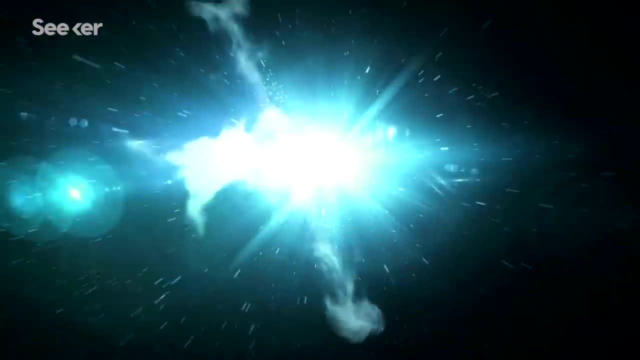 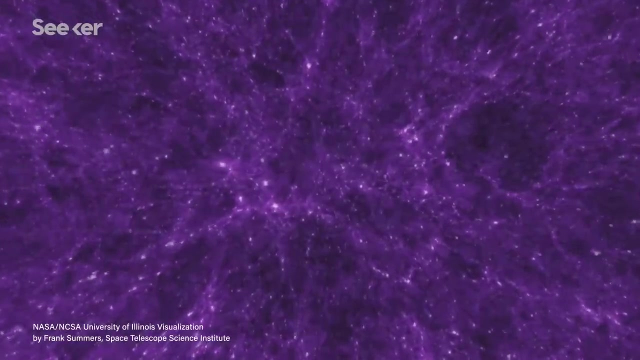 and the only side effect is there's this extra particle called the axion, And it's produced in large amounts in the early universe and doesn't interact very much. so it's still there And so it's just as a consequence of fixing this nuclear physics problem. 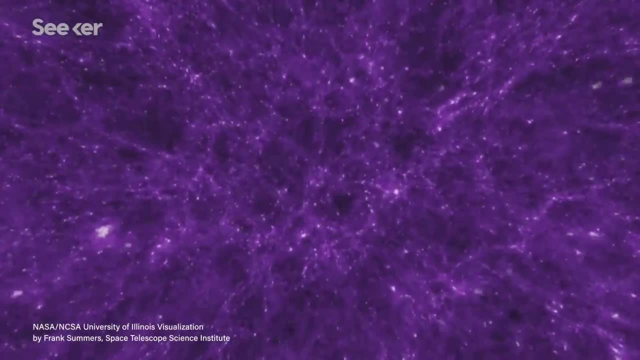 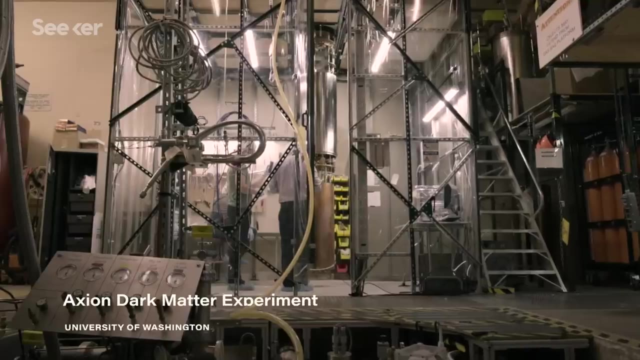 you have stuff out there gravitating, not interacting, and it fits the bill for dark matter just perfectly. It's too good of a coincidence to not pursue, to not go and try and find the axion. Okay, so how do physicists set out to find this hypothetical particle? 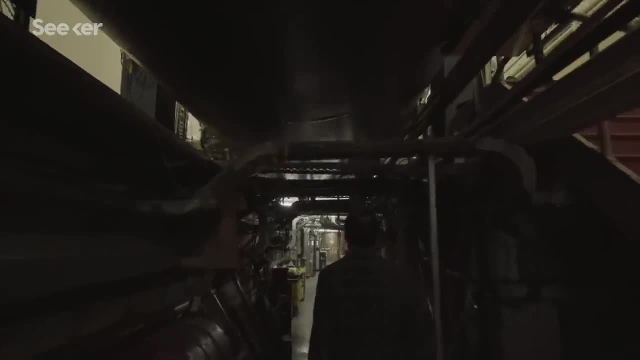 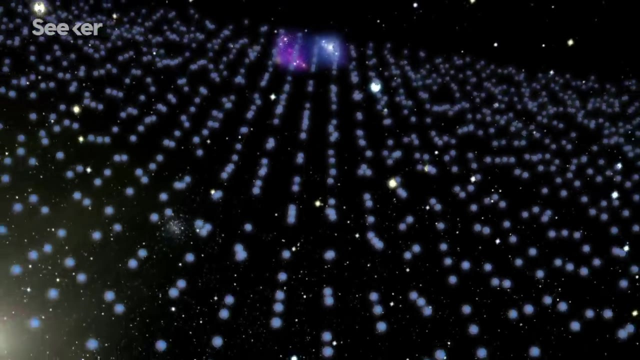 that may or may not exist. First, follow the theory. It's almost certainly very light, and when I say very light, much lighter than an electron Being light actually makes it much more wave-like than particle-like. It would act a lot like a radio wave. that carries a little bit of mass. With the right conditions you can convert energy between axions and real radio waves, and basically you just need a strong magnetic field that can do this conversion process. Then build an instrument that's specially designed to do this. 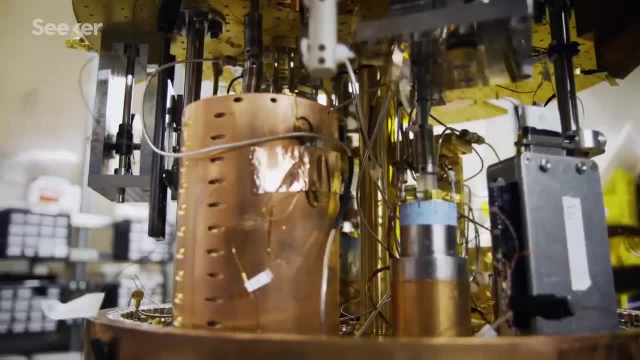 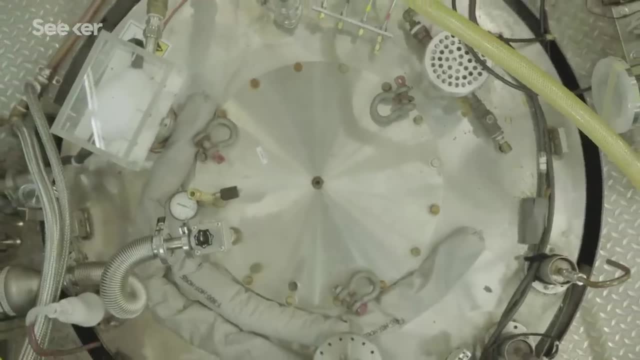 called a haloscope. It's basically a telescope, but looking for the dark matter halo. The whole experiment sits in a large magnet around 8 Tesla and that promotes the conversion of axion dark matter into detectable radio waves. We do this inside a microwave cavity. 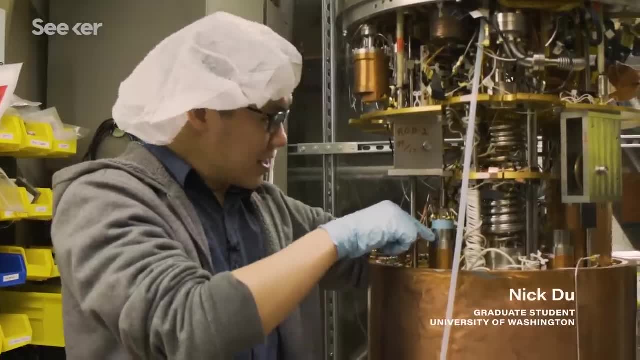 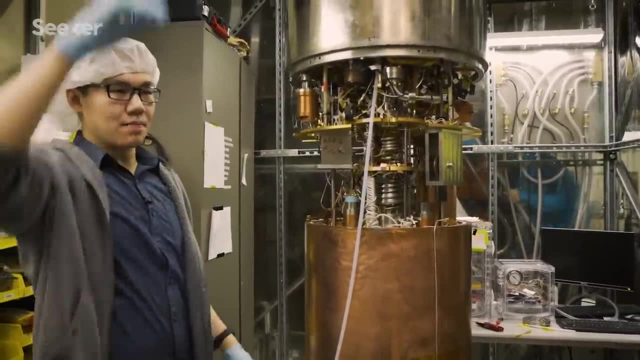 which is like a big soda can made out of copper. The cavity itself is actually tuned by two tuning rods. Those are positioned here and here. They're connected all the way to the top by a couple of gearboxes and the idea is that within this cavity, 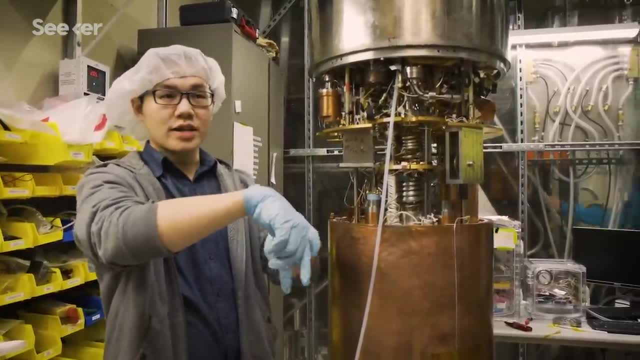 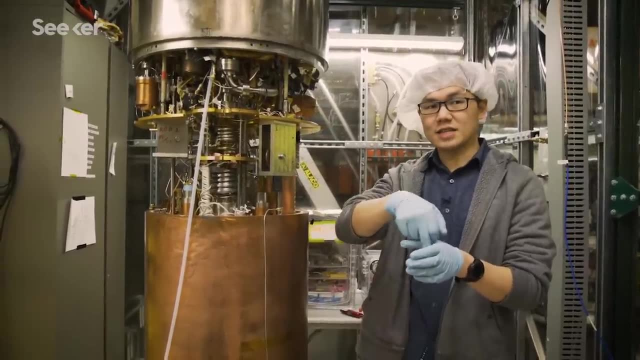 you move the tuning rods slowly like you've had to tune an AM radio, and you tune the resonant frequency of the cavity. This little doohickey right here is the actual antenna. so that's what we put into the cavity to actually pull all of the power out. 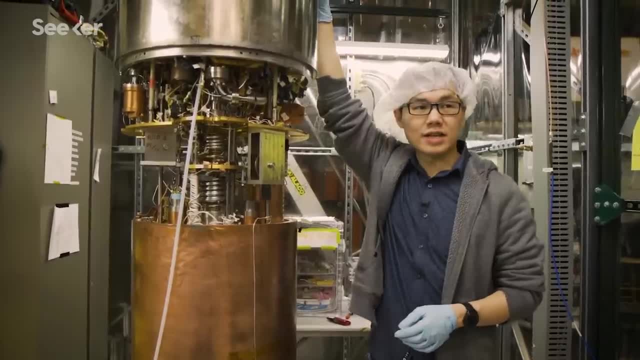 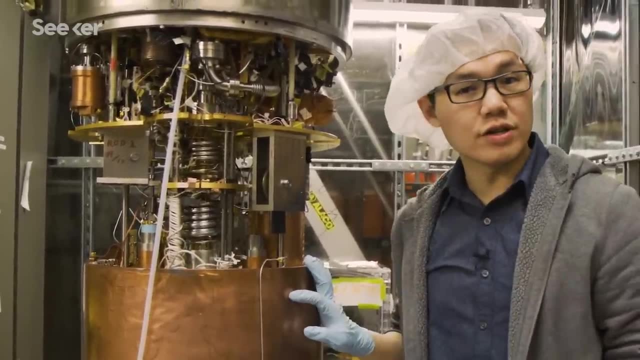 There, all of that power gets sucked into something that's kept stored in here, which is called our quantum amplifier package. The whole thing is kept cool by this right here, which is our dilution refrigerator, Because axion interactions are so weak. 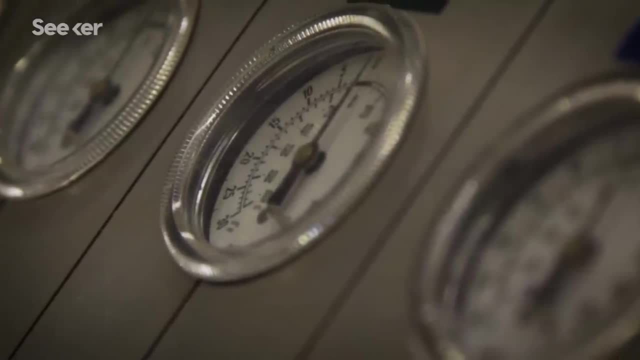 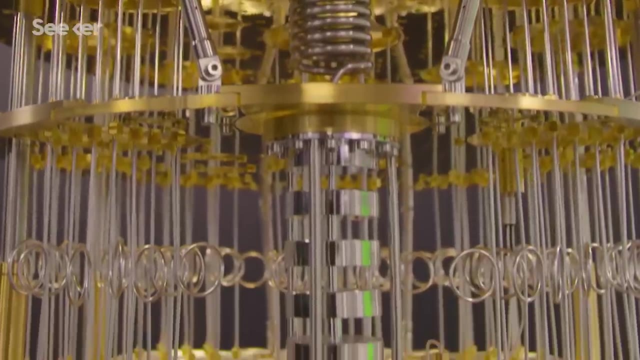 You need almost no background, and there's plenty of background just from things having a temperature. They just radiate, And so you need technology to make yourself get very, very, very cold, And that's where we've tied in a bit with quantum computing. because quantum computing involves making measurements at the bounds of quantum mechanics. There's been a lot of development for radio-scale amplifiers and ultra-sensitive electronics that work at these ultra-cold temperatures. So while they're trying to read out their qubits, the same sort of devices can be used. 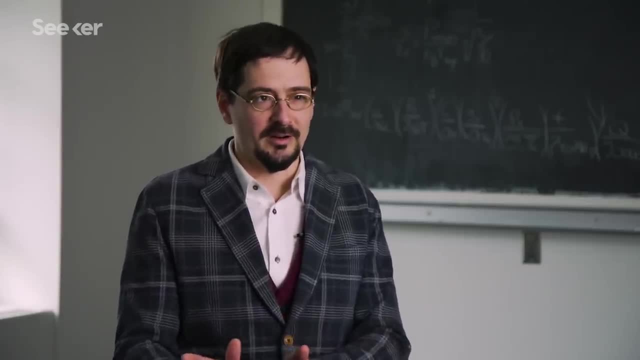 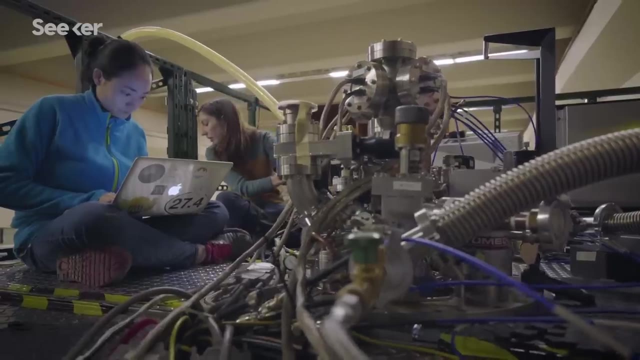 to try and detect extremely small amounts of power that might be coming from dark matter. And the difficulty is, I said, oh, you want the cavity to be at a particular frequency that corresponds to where you want to look for the axion. That frequency has a lot of wiggle room. 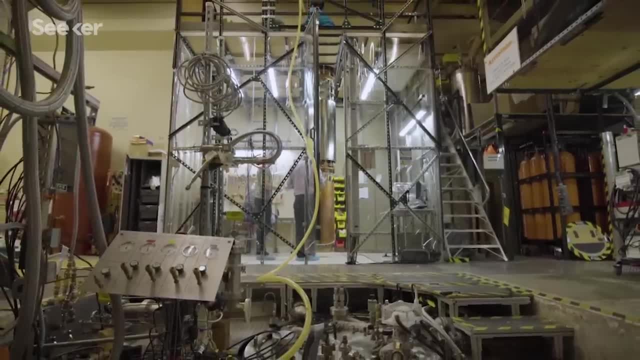 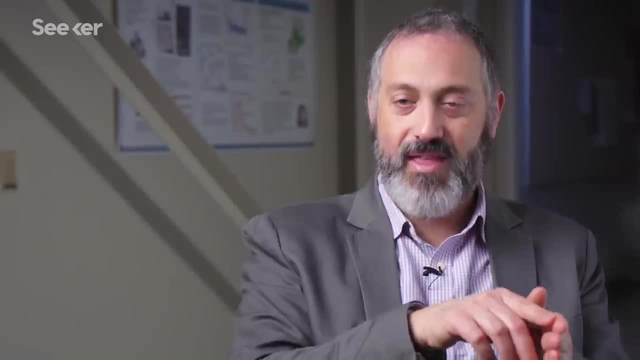 according to theorists. So we'll start around 500 megahertz and working our way up to, say, 10 gigahertz. So we'll look at one region, one frequency range- We'll not see any power out- And then we move on to the next range. 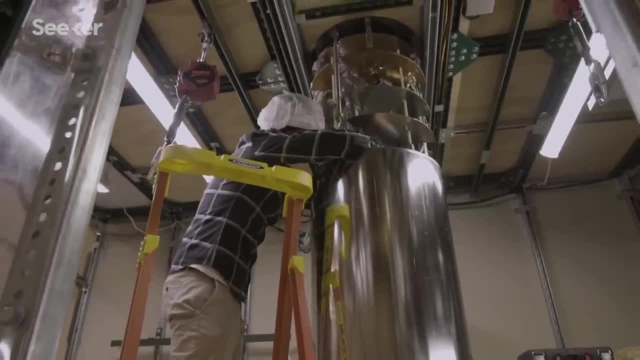 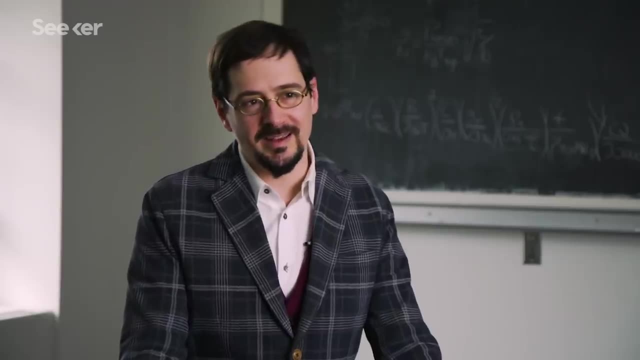 and we have to be able to scan that very quickly. Most of the work is in just keeping the experiment running. It has many moving parts, many complicated systems. They all have to be maintained. When they break, you have to fix them. 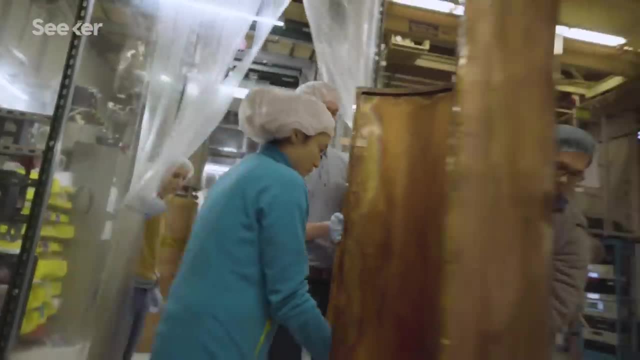 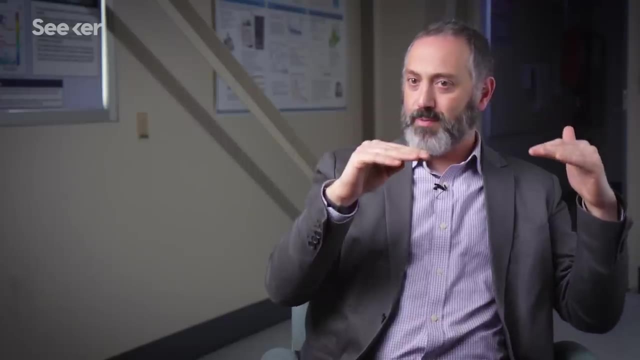 Which is exactly what happened when we came to visit. This is a persecuting issue with doing stuff in cryogenics. We're sending signals through the system As we cool down those power levels dropped, which doesn't make any sense. We're trying to diagnose what we think is a fault in the line. 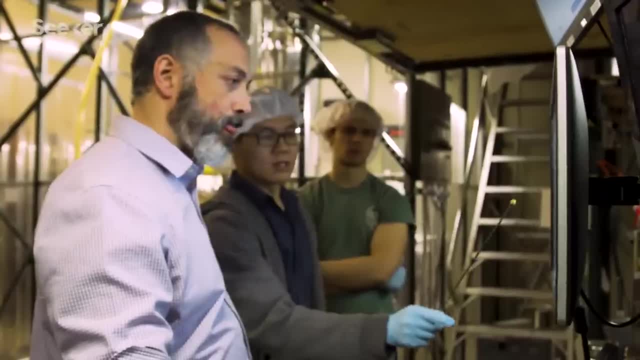 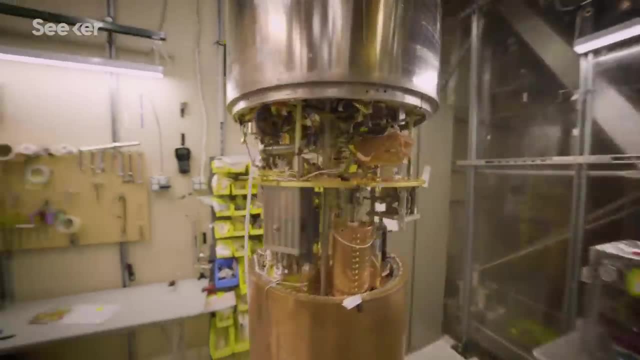 And this is a very critical cable that's coming out of our experiment which would measure power from the axion, if an axion were to interact in our magnetic field. There are experiments that have many thousands of cables and you don't want to go through and examine them all by eye right. 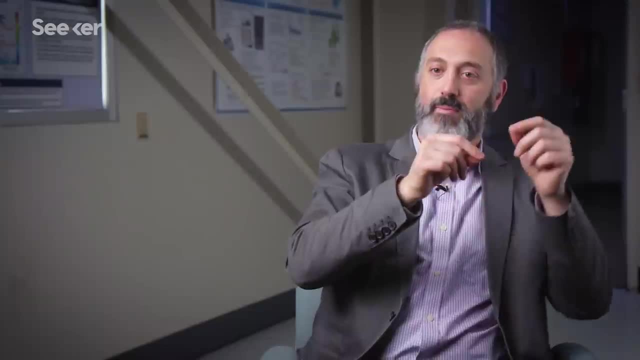 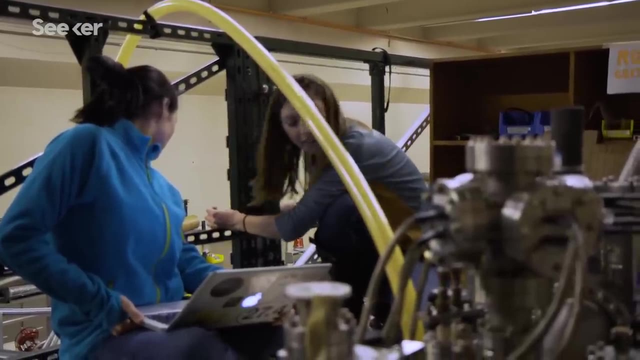 We'd do a measurement. We'd take the next cable off, do a measurement So we could measure the point where we actually got to where the error was. I think he just disconnected it at the top. Oh, At the top. That's interesting because I think that's where the break is. 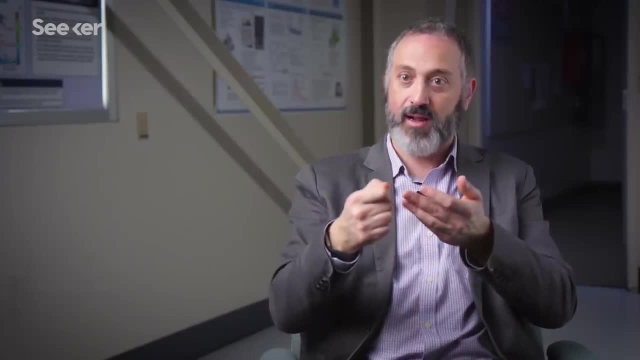 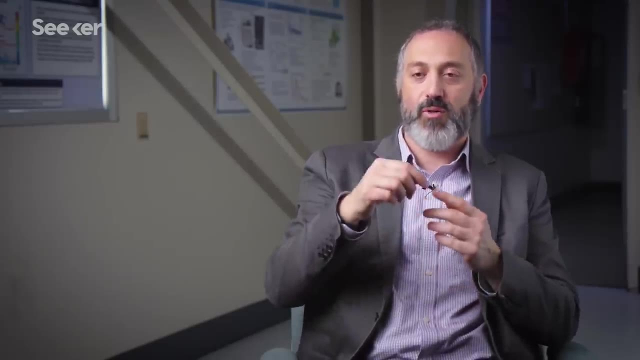 Just looking at this, Due to strain on the cable, part of the pin actually just pulled back. Things strain and contract when things get cold And so that caused this little gap to appear. We would not have been able to take good data with that. 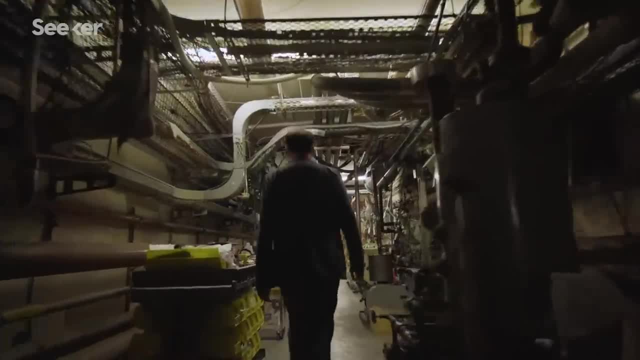 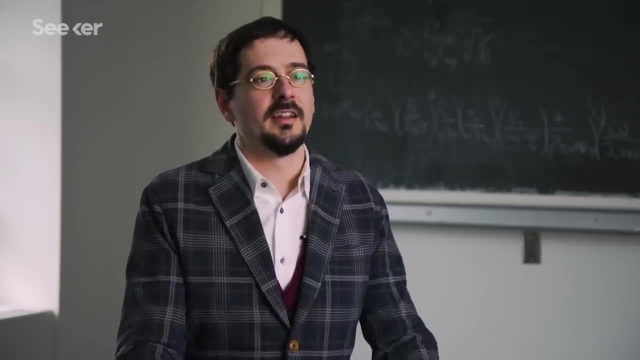 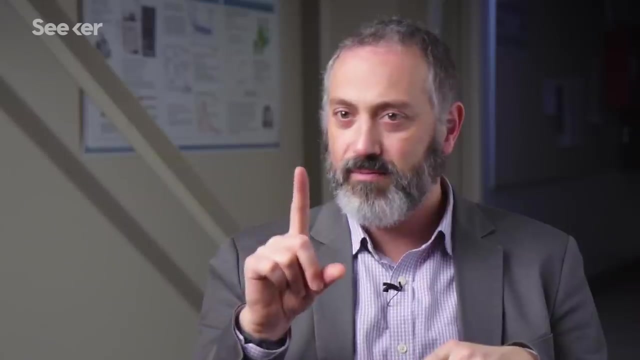 We've recently crossed the threshold where we are now sensitive to the types of interactions the theorist predicts for axions. Kind of the exciting thing is that any day you could just hit it and it's there and it'll be obvious and clear. My dream is that I get a call or I'm looking at the data and I'm like there's a little. 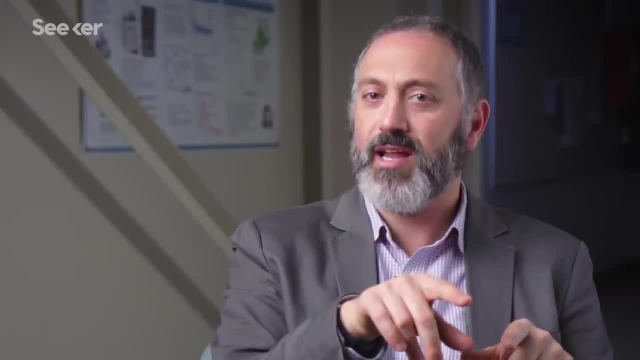 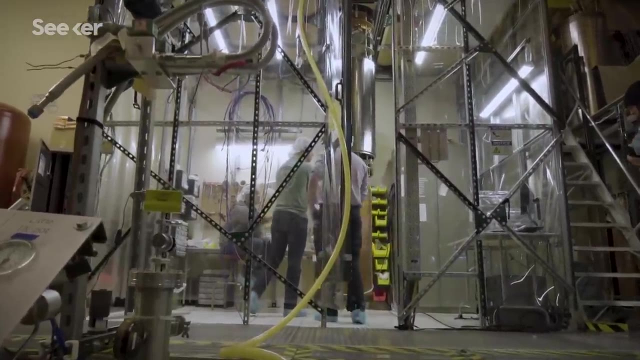 peak there. Let's zoom in on that. let's take a little more data on that. Oh, that peak is staying there. Let's move that magnet down. But so far, by and large, it has been white noise. The axion parameter space is quite wide and unexplored.